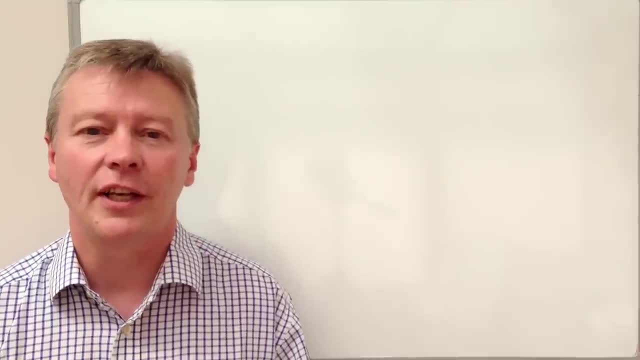 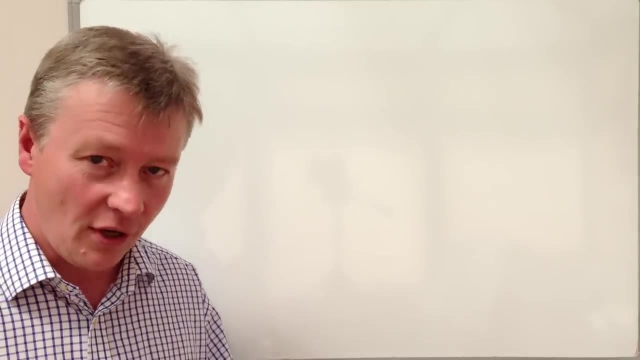 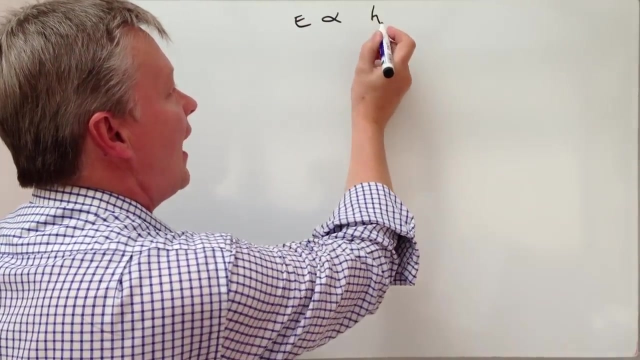 within direct proportion, Or you can have a look at the post on mathsrapcouk. What we really talked about, and the example I used, was earnings. What we said was that earnings is proportional to the hours that are worked, and we used a particular term which is called. 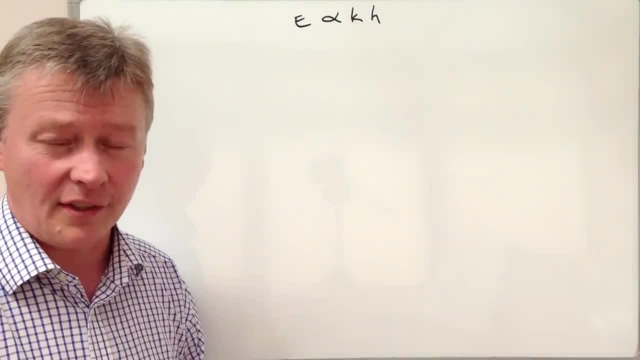 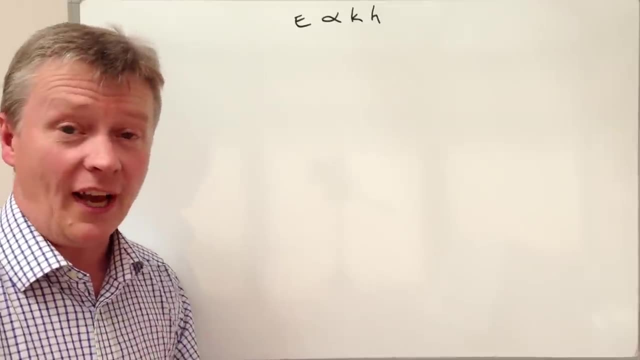 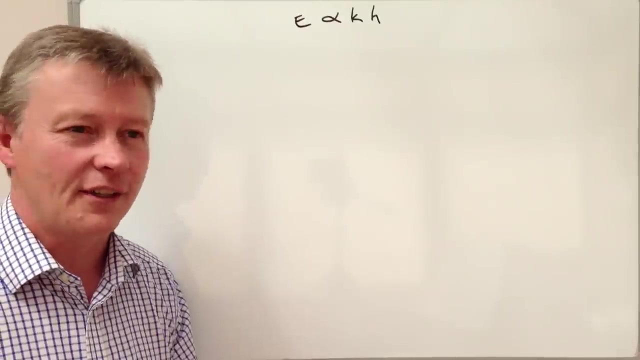 K. Now that K is constant. so in this particular formula, your earnings are proportional to the amount that you're paid, and I think the example I used was in the UK, maybe £8 per hour, and I think I said something like $15 per hour for America. This is direct proportion. 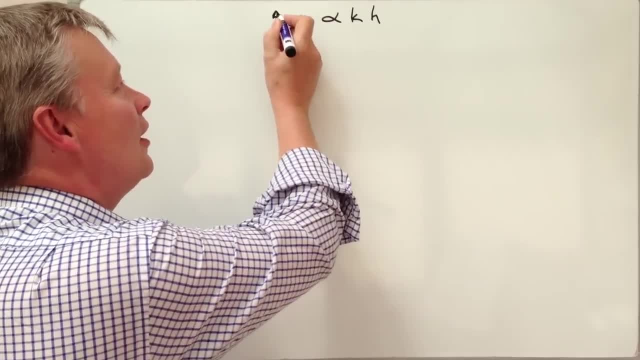 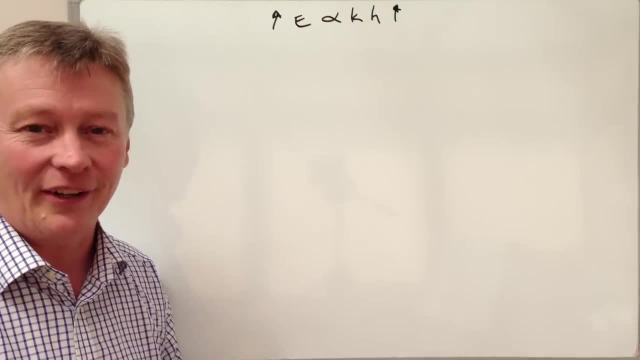 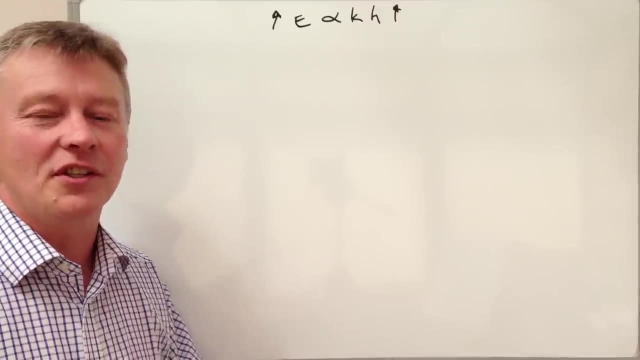 which basically means that your earnings will go up the more hours you work. so there's a direct relationship to it. The video today is going to be looking at the difference between direct proportion and direct proportion. I'm going to be looking at inverse proportionality, In other words, there's still a proportional. 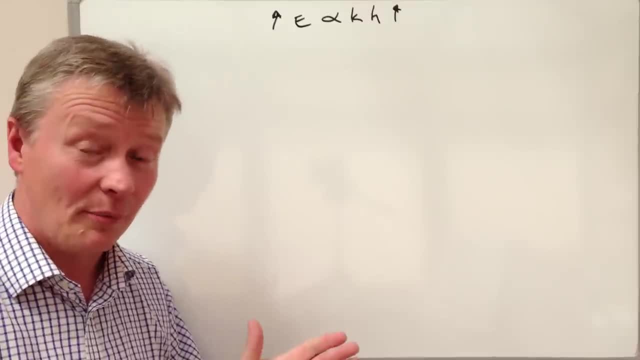 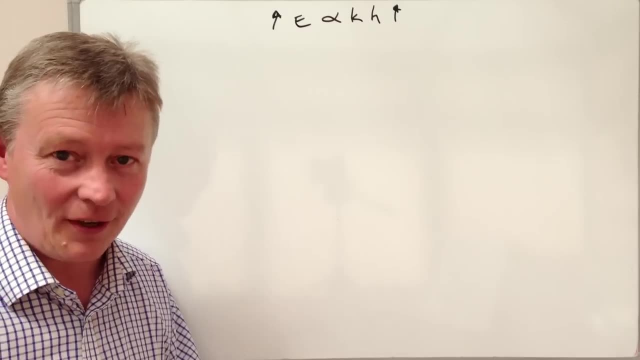 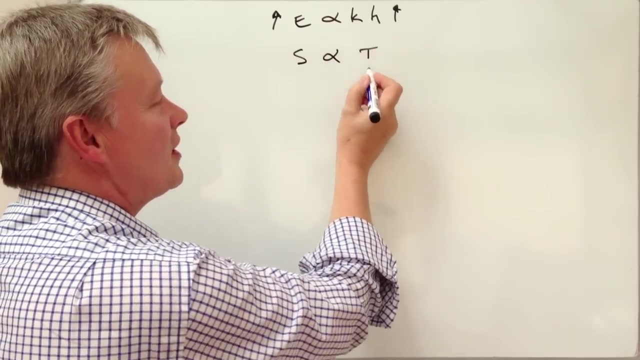 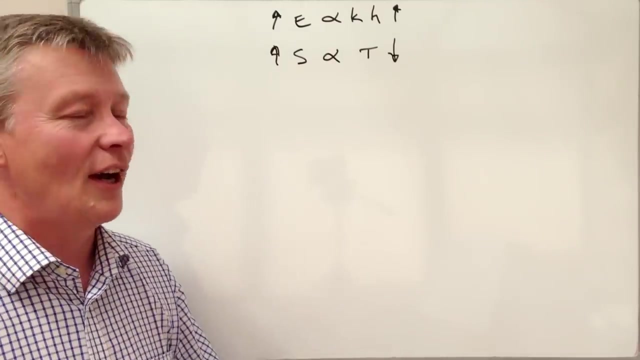 relationship, but as one side goes up, the other decreases by the same rate. So a good example of that will be speed and time. So, for instance, if I have speed, it is proportional to time. but as speed increases, time decreases. So, for instance, if you're 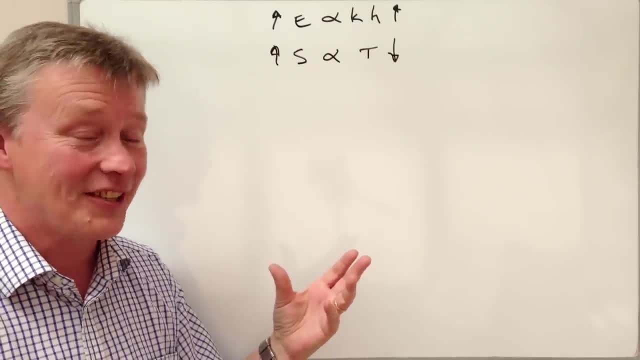 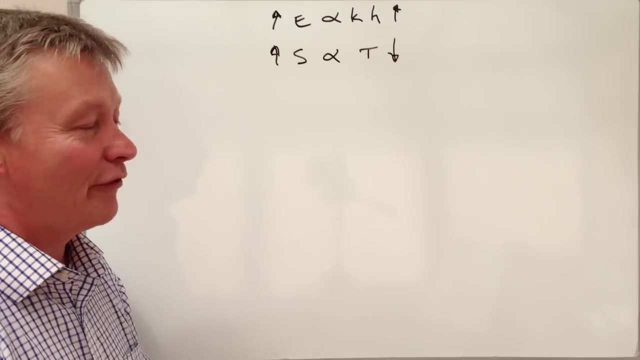 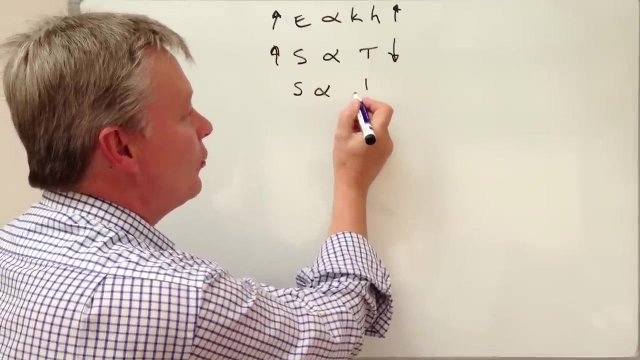 driving somewhere and you drive somewhere very, very fast, then the time that it will take to get there will be consequently reduced. Now the way that we write that for inverse proportionality is speed is inversely proportional, which is 1 over t or 1 over time. 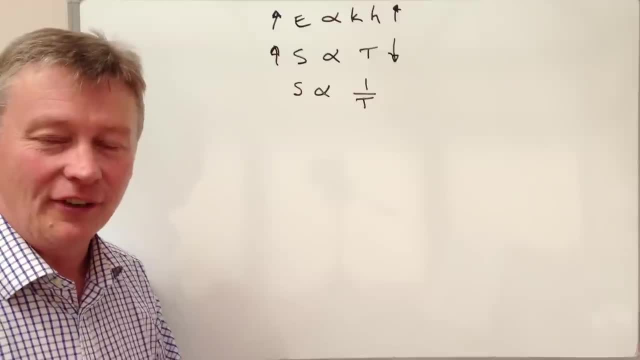 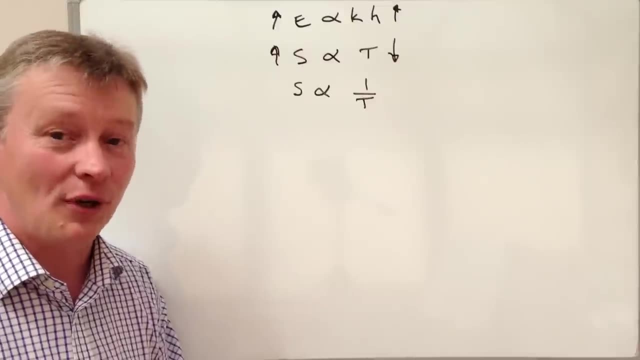 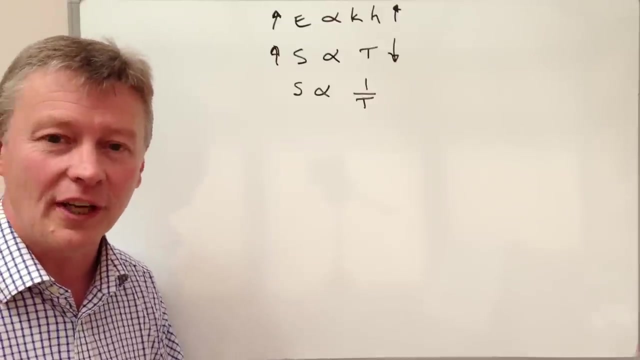 Okay, now I'm going to give you an exam question. It's round about 8.5.. I'm going to give you an A grade, B grade question. I will write it in the description box underneath and that will give you something to refer to or you can have a look at mathstrapcouk. 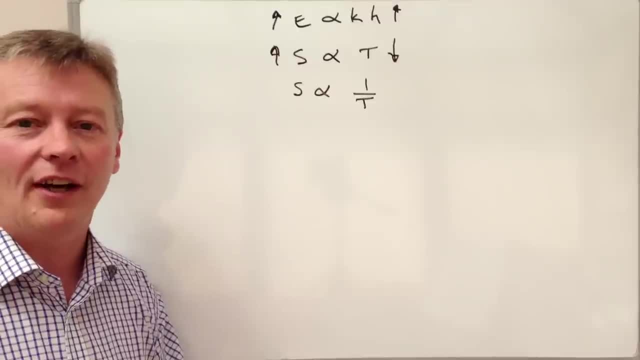 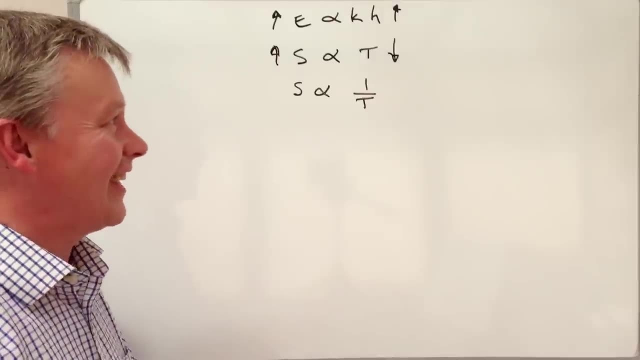 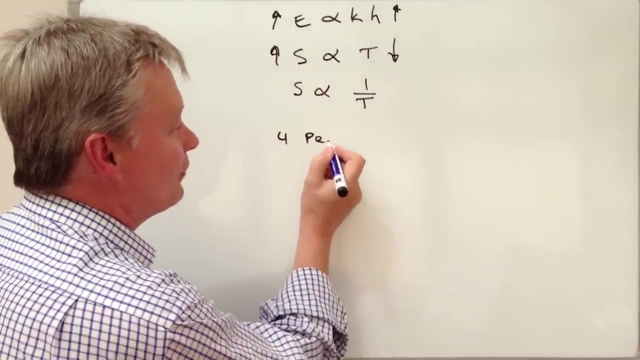 If you do, there are some quick tests that you can download and have a go at them for yourself. Okay, so this particular question deals with painting a fence, alrighty, and the question that's given to us, or the information given to us, is that it takes four people to paint. 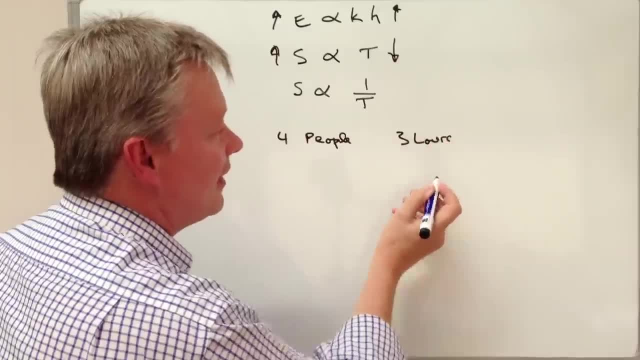 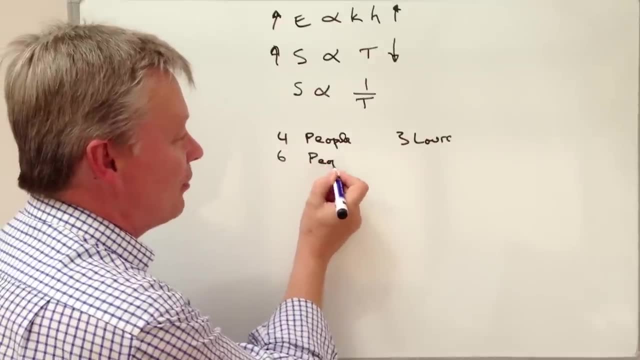 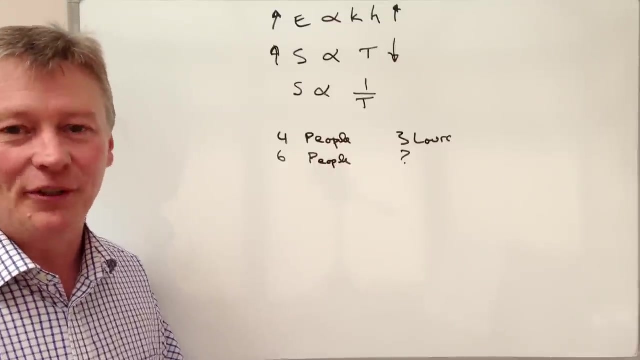 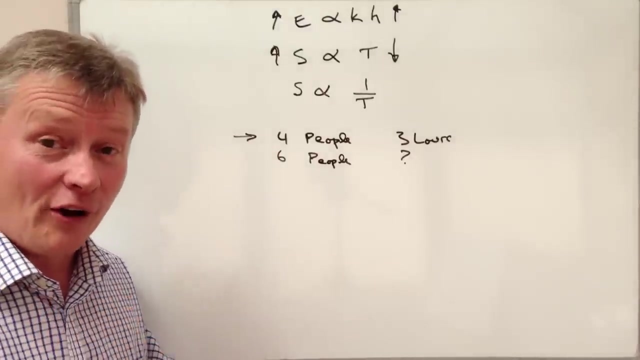 a fence. Three hours to paint a fence- okay. The question is: how long will it take six people to paint the same length of fence? Alright, this is a fairly typical inverse proportionality question. The first bit of it will allow us to work out the value of k, which is the constant. 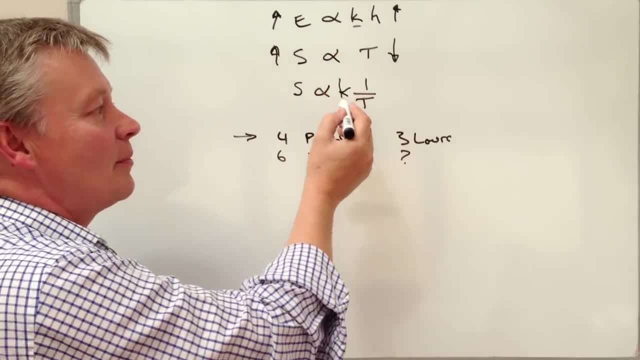 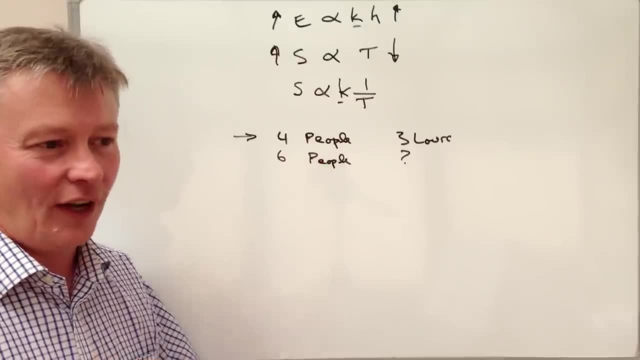 It's this bit that goes in there. Okay, This bit goes in there or this bit up here, and basically it's the rate at which the four people work. So it could be the amount of fence panels that they're able to complete in a fixed amount. 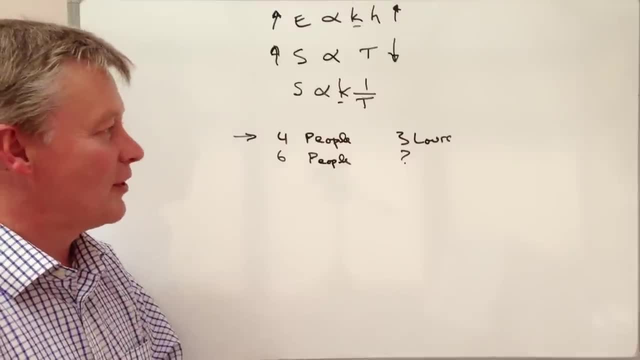 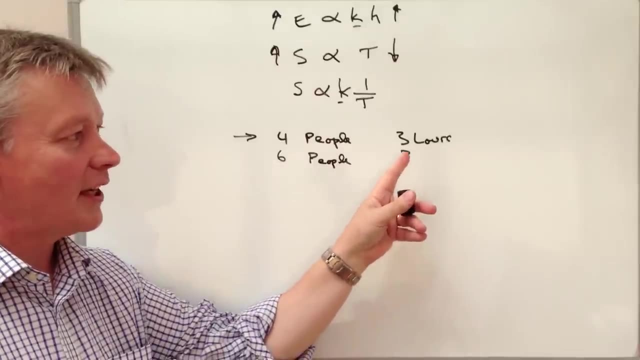 of time- in this particular case, three hours- and what we're going to do is work out this value of k and then use the value of k in order to find out how long it will take the six people to complete the same job. 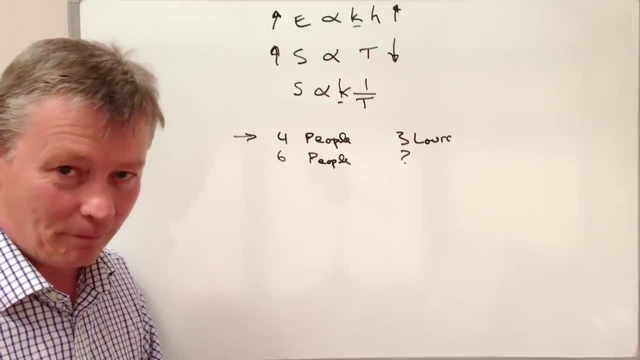 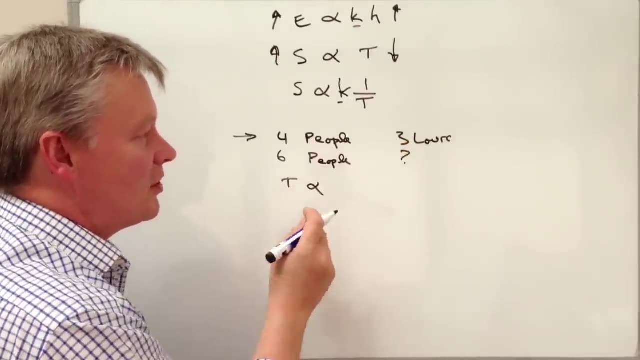 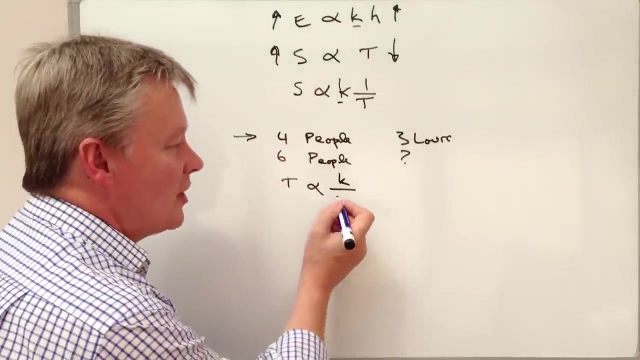 Okay, So the information that we're looking for. What is time? Well, as we are at the moment, time, which is this three hours, is proportional to the rate at which they work and it's inversely proportional to the four people. 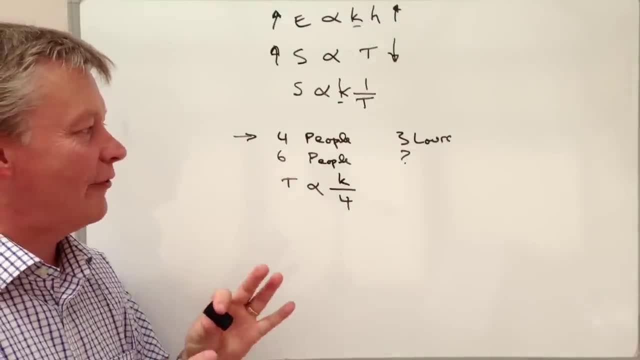 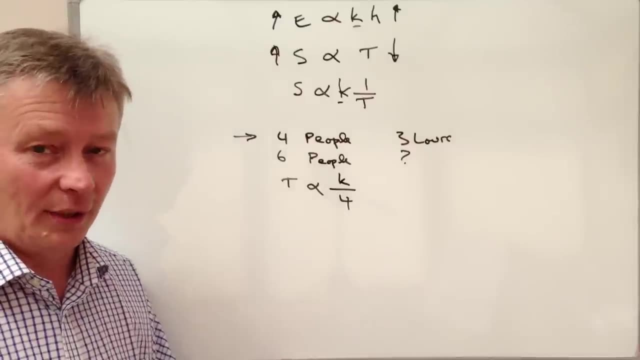 Okay. So I think it's just a little bit careful that with these sorts of questions you've got to work out whether it's inversely proportional or directly proportional. Sometimes the clue is in the question. Okay, Sometimes the clue is in the question and it'll tell you. 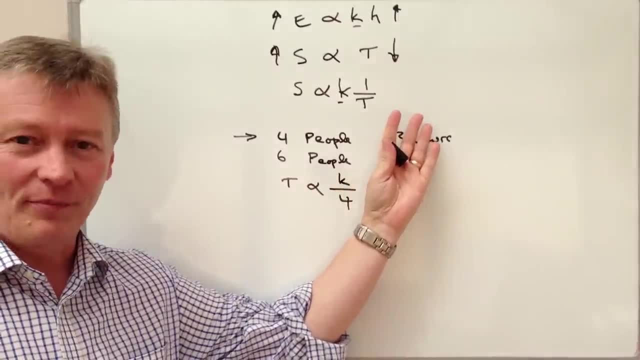 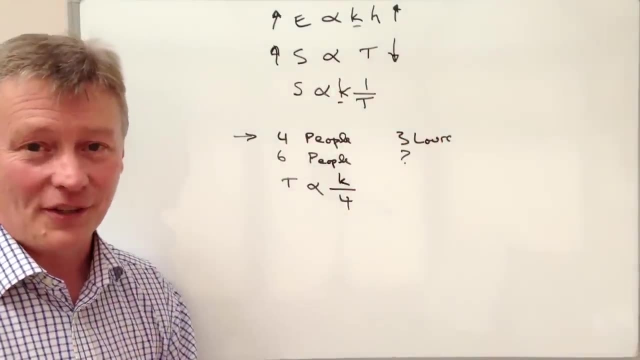 Other times you need to kind of look at it just as four people to do a job, six people to do a job. So therefore it's going to be a quicker amount of time in which to complete, in this case, the fence panels. 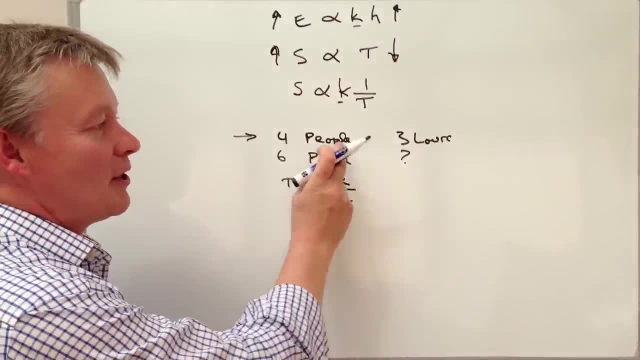 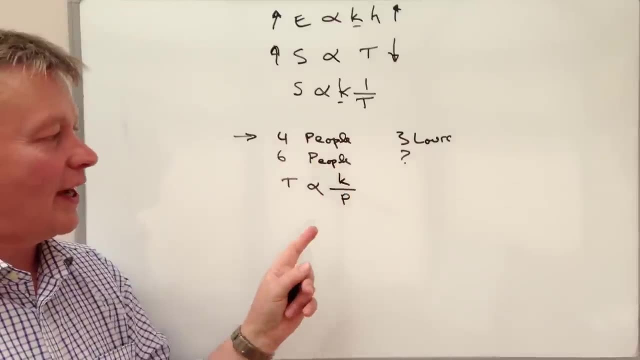 Okay, So what we need to do using this information- the four people and the three hours- is- I'm just going to make that p, actually the four people and the three hours- is work out this value of k, And I'm going to use that in the next little bit of the question. 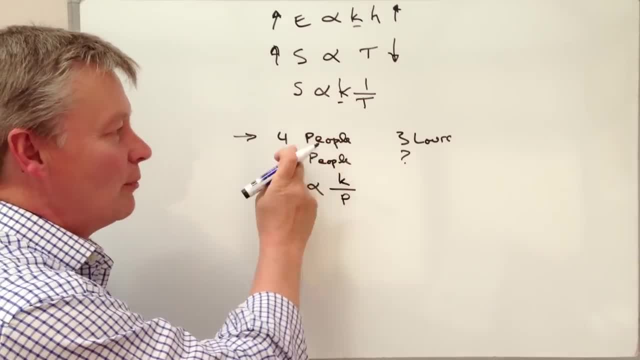 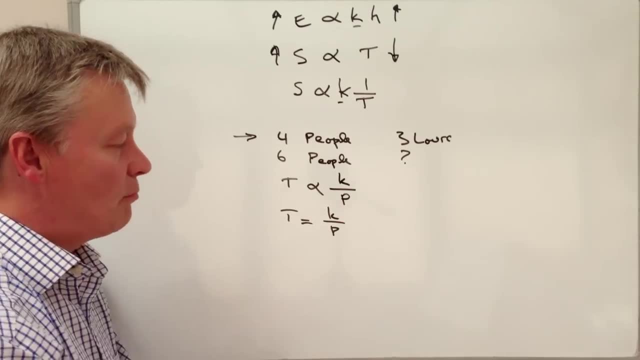 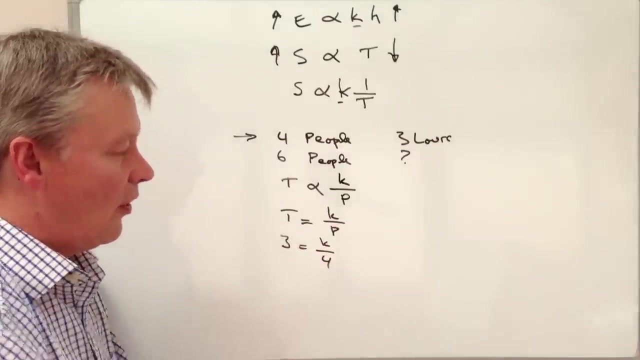 Okay, So let's put the numbers in. So at this particular moment, the four people and three hours, then t equals k divided by p. So the three hours equals k over four, And if you use a little bit of algebra to manipulate that, you can work out that by: 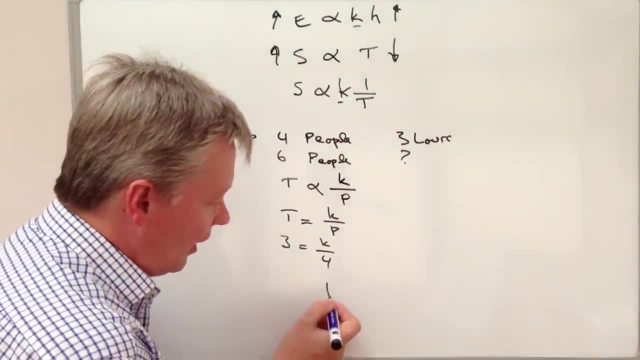 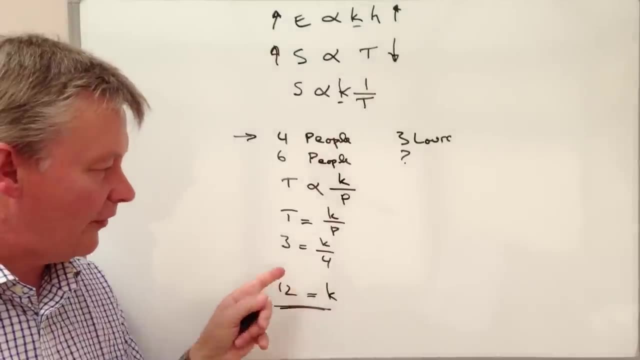 multiplying both sides by four, I can work out that the four people and three hours is equal to k divided by p. So we've got the value of k as being equal to twelve. Okay, If you're not sure about that step, you need to perhaps have a look at some of the algebra. 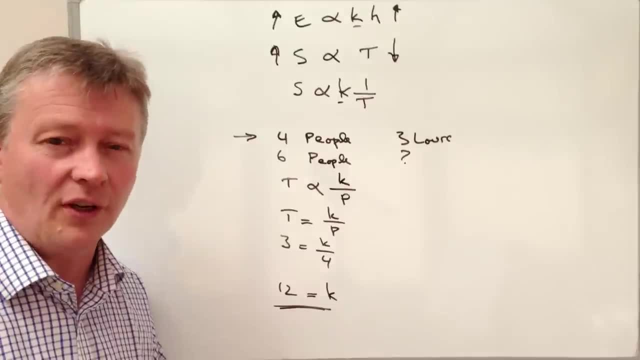 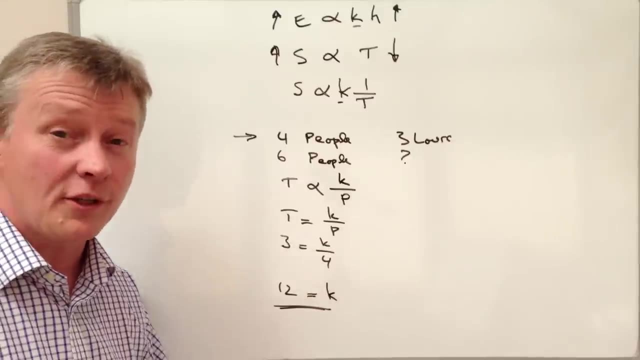 videos on the YouTube channel or do a quick search on the MathStrap website, and that will give you some detail about algebra and how we balance algebraic equations. Okay, So the value of the rate of work is, in this particular case is, twelve. 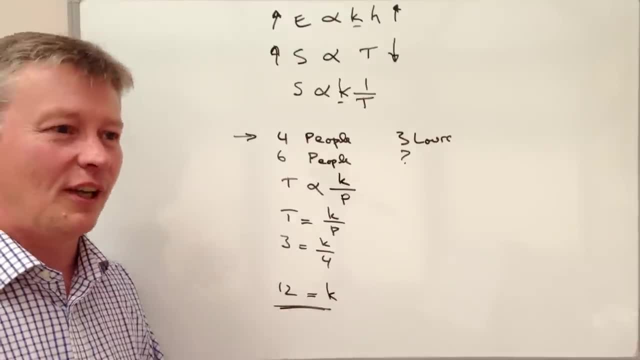 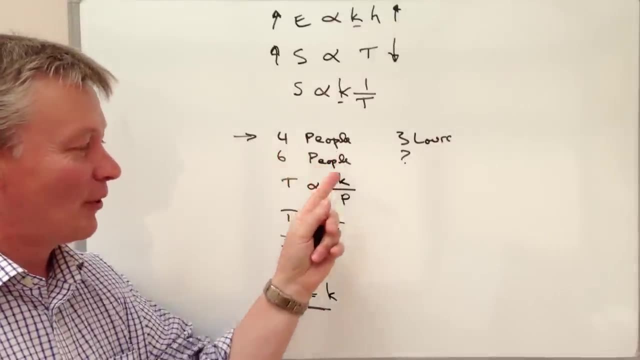 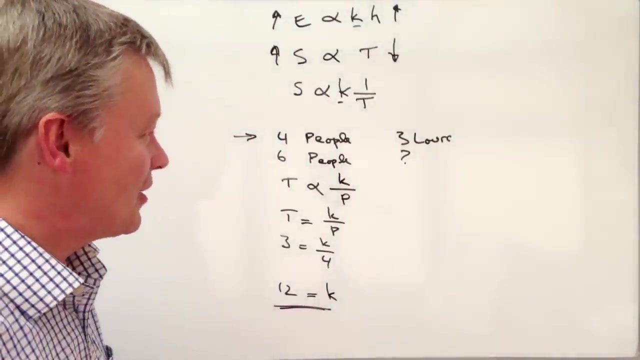 So it could be twelve panels, panels, or it could be 12 fence posts or sticks or whatever it might be, I don't know, But it's taken these four people three hours, a rate of 12, let's say, panels per three hours. Okay So 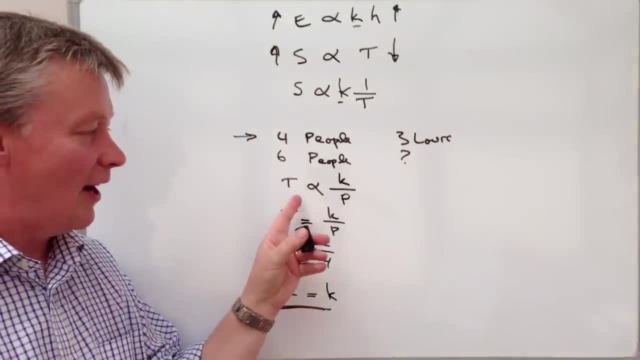 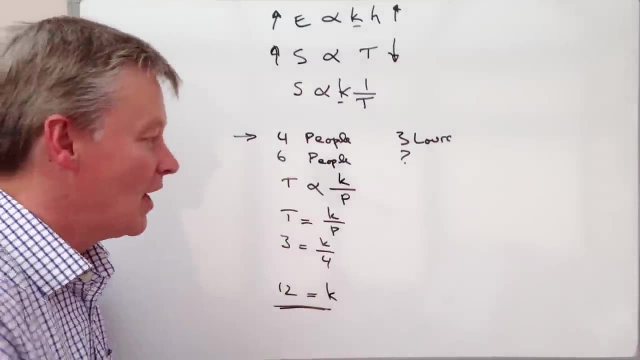 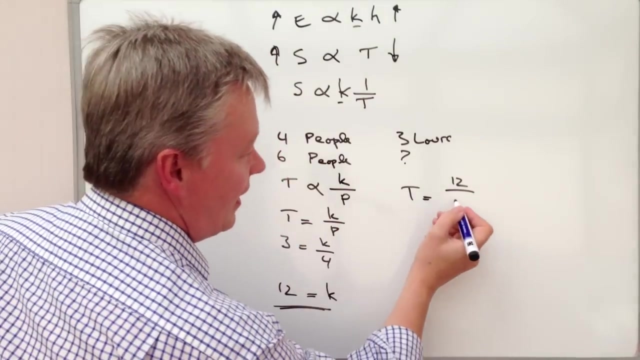 we're going to use that information and we're going to put that into the same formula, but this time we have a value of k and we're going to work out the value of t for time. So t equals k, which is 12, divided by 6 in this particular case. So, in order for us to find out the value, 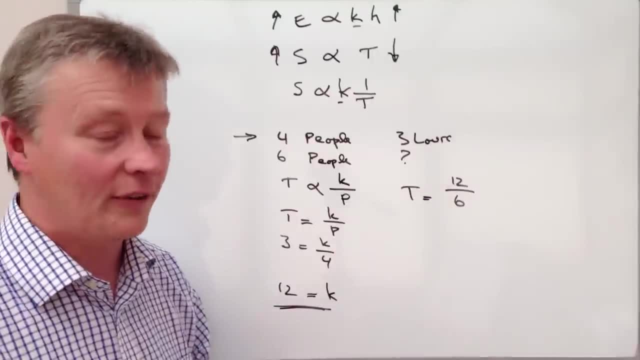 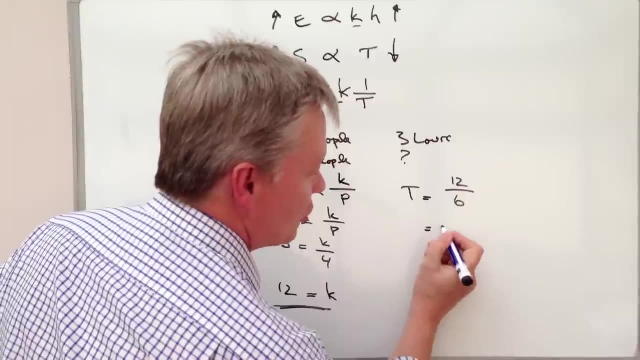 of time it's going to be. k is the 12,, so 12 panels. but it's going to take six people this time to do the same 12 panels. So 12 divided by 6 is 2.. So it's going to take two hours for. 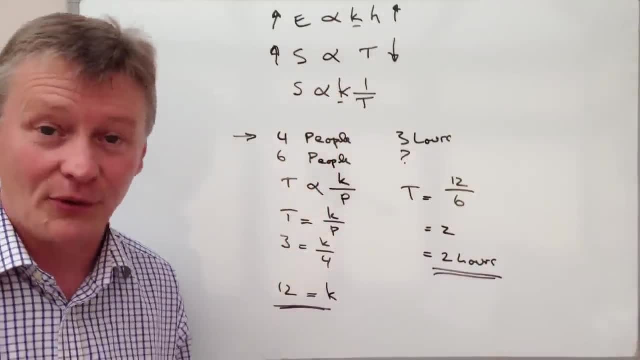 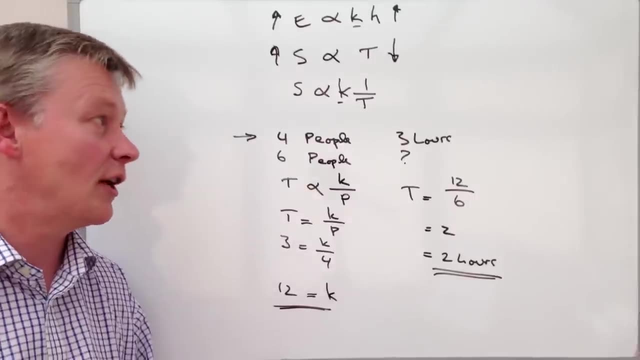 six people, And that would be the answer to your question. I hope that's okay. I will write the whole question in the description box on the YouTube channel Or you can have a look at the MathsRamp site and there are some quick tests for you to. 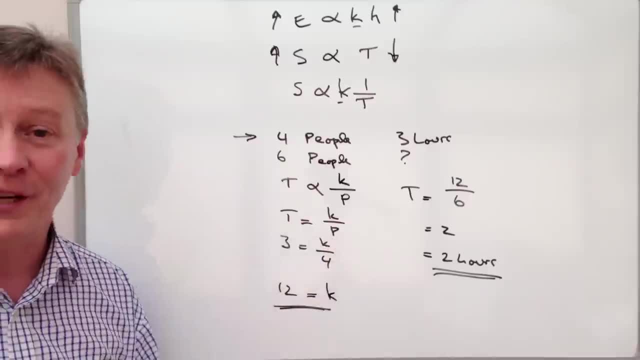 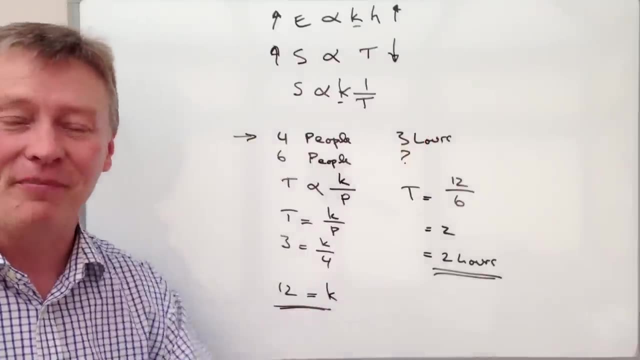 have a go at for yourself. Thank you very much for your time today. I hope it's been useful to you. Please do post, pin tweet this particular video. You can subscribe and you'll be posted the next time I post something And I'll look forward to seeing you inside the next video. Have a great day. 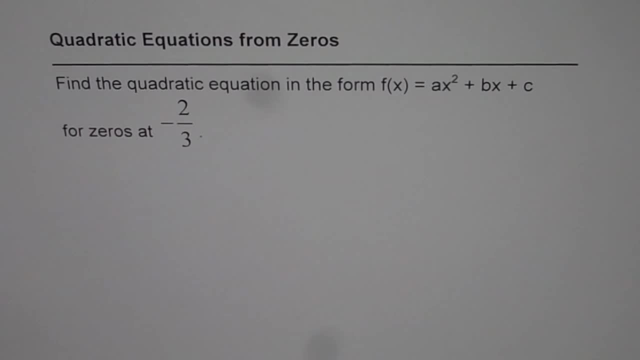 In this video we will learn how to find quadratic equation from given zeros. Find the quadratic equation in the form of f of x equals to ax squared plus bx plus c, for zeros at minus 2 over 3.. So we need to get a quadratic equation and we know only one zero. It simply means: 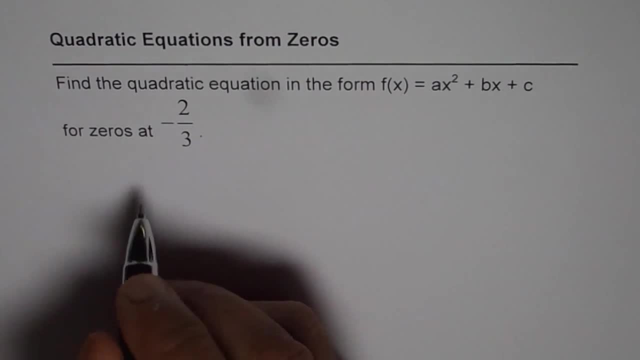 that we have a double zero at minus 2 over 3.. So if we have a zero at minus 2 over 3, that means we have a factor. at which point Factor should be 3x plus 2, right, Since this. 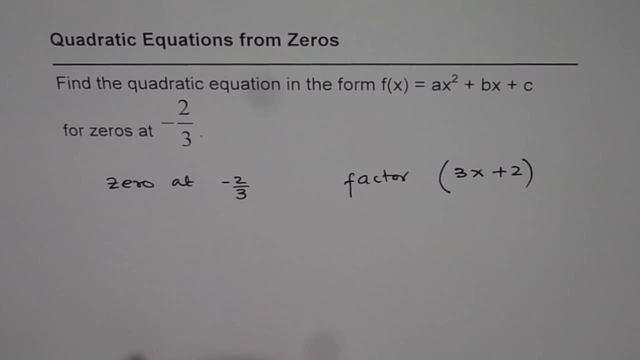 factor will be zero, for x equals to minus 2 over 3.. You get the point right Now. as we know, it is a factor of a quadratic equation. It simply means that we have two zeros, We have a zero of order 2, right. 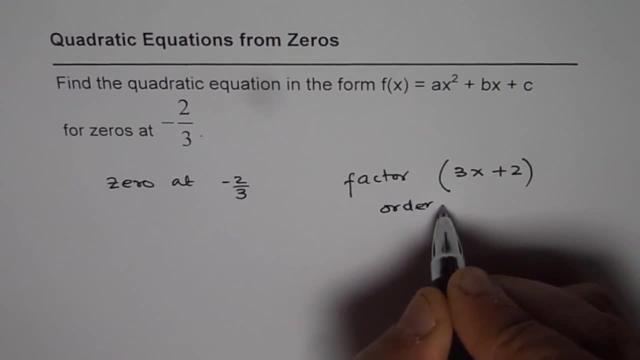 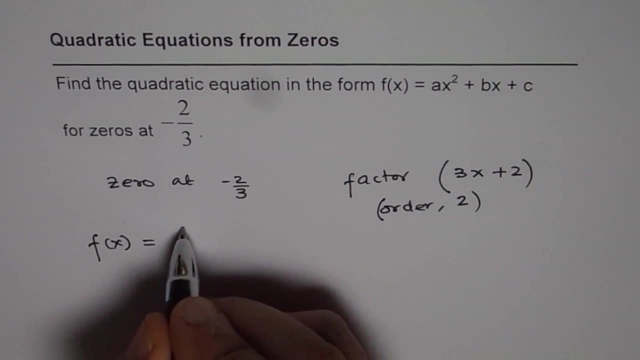 So this zero is of order, or sometimes we say multiplicity order 2.. That is to say that the function which we want to figure out is basically 3x plus 2, whole square, right. So we can always expand this and find the quadratic equation in standard form. So we get 9x squared. 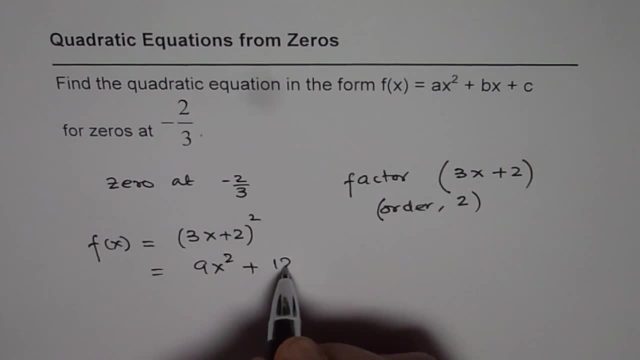 plus 2 times ab, that is 4 times 3, is 12, x plus 4.. So that is the answer. This particular equation, quadratic equation- will have a zero at minus 2 over 3.. So that is how we.